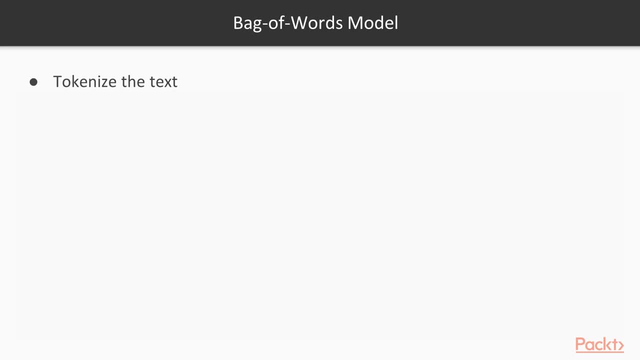 given that we want to analyze or do some predictive analysis on like sentiment analysis, we tokenize the text. basically, tokenization means extracting the words out of text, which is usually done with spaces as boundaries. once we have the words, we identify the unique words and that constitutes our vocabulary. so we 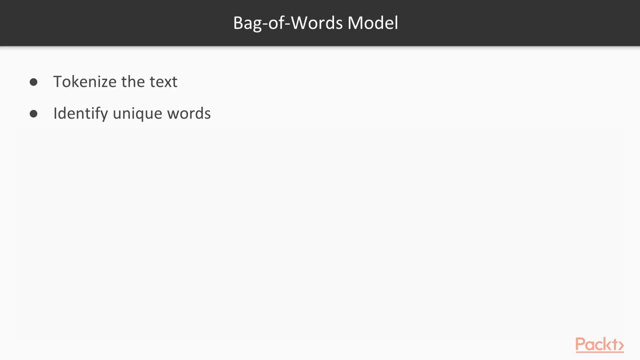 might have, for example, a piece of text where a total of hundred words are used, so those hundred words are our vocabulary. then we count the occurrence of each word in our vocabulary within the text and that constitutes our bag of words. and then, once we have this representation of the text as a bag of 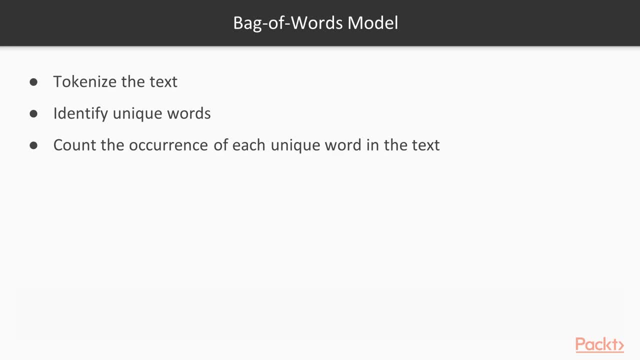 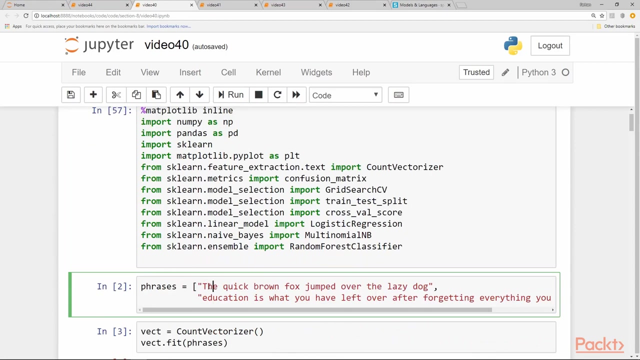 words, meaning, unique words and their counts. we can use this representation to apply a different machine learning models on it. so let's see how we can do that. as usual, we import a bunch of libraries. we start with a simple example of two phrases stored in a list. so this is the first element of the list and 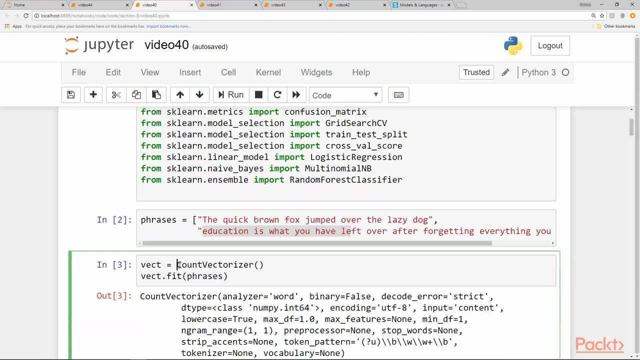 this is the second element. scikit-learn provides us a class called count vectorizer which implements the bag of words model. we create an instance of the count vectorizer and we fit our phrases- list of two phrases- to the count vectorizer. so it creates an object and it fits the data and it also. 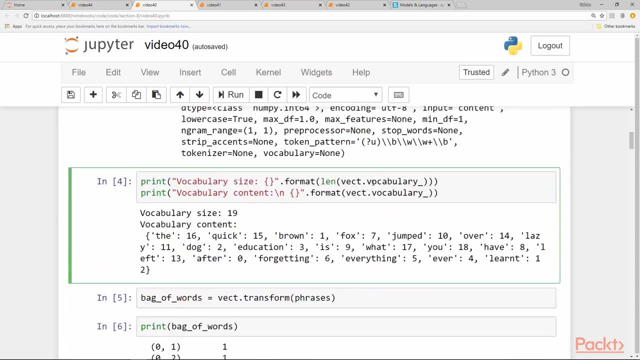 creates a vocabulary while fitting the vocabulary is contained in vocabulary underscore field of the vectorizer object which has been fitted to the text, and it is size 19. so there are total of 19 unique words in our vocabulary and the content shows us a dictionary where there is each word with its assigned index. so 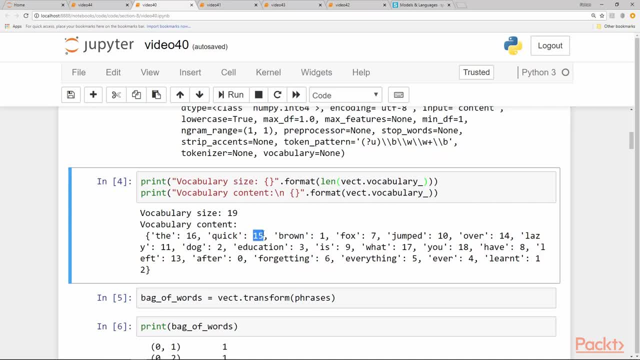 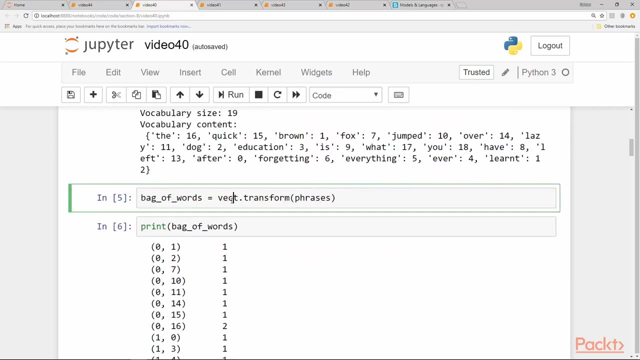 the has been assigned index 16. quick has been assigned index 15. so each word in the vocabulary in the bag of words model is represented by an index into an array or a list where that words count resides. the next step is to transform the phrases using the fitted model so that we get our bag of words. bag of words. 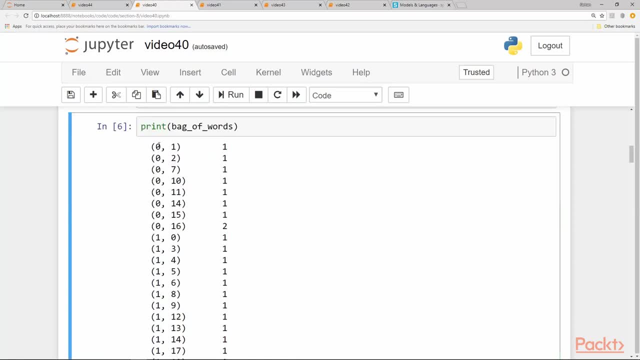 looks like this. we have these tuples. the first element is the training example number. well, so we have only two. so 0 and 1 are the indexes of the training examples, or rows of our data set, and the next element is the index assigned to the word as part of the vocabulary, and then it is followed by the count of the word. 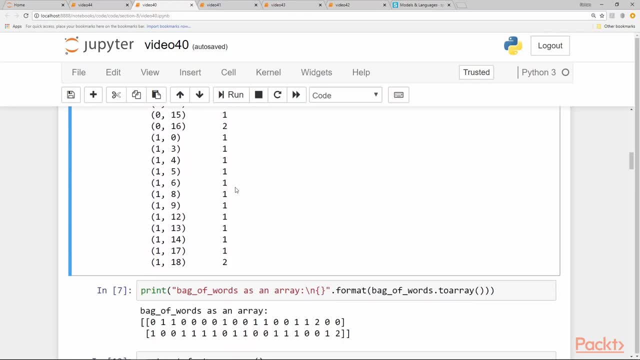 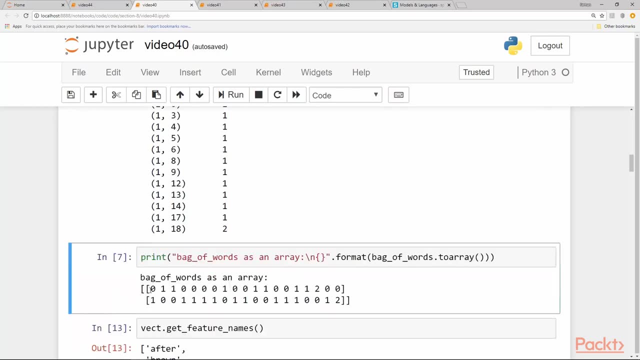 in the corpus or in your text. so if we convert our bag of words into an array, we can use the to array function is something like one hot encoding. so we have the full vocabulary here. so for the first phrase, full vocabulary. all the 19 words which are here are represented either by: 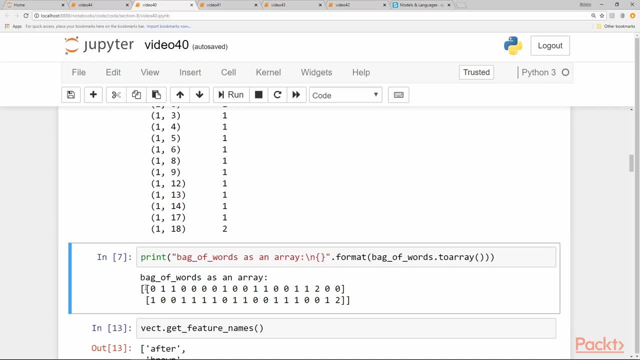 0 or by their count. so in the first sentence the word at index 0 occurs 0 times and the word at index 1 occurs 1 time, the word at index 2 occurs 1 time, and so on. this is index 16 if you count from the start. so we: 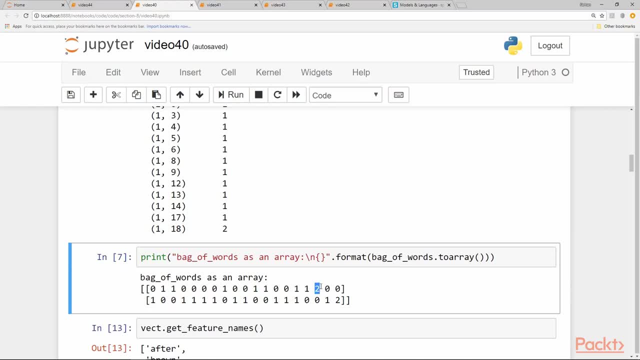 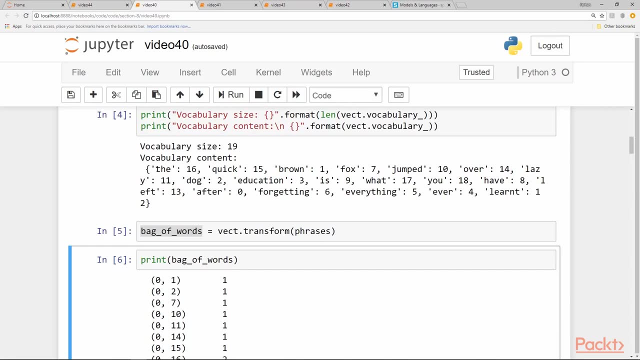 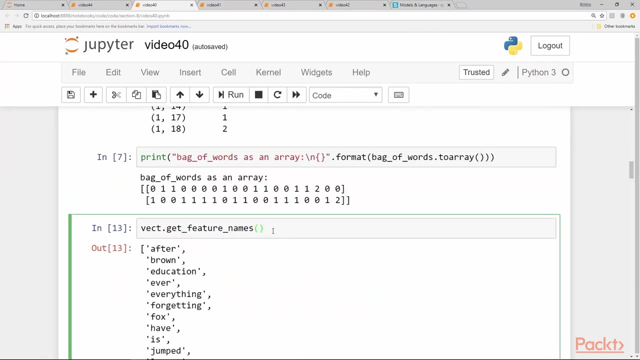 have indexes from 0 to 18 and this is index 16 and, as you can see, index 16 occurs two times and in our vocabulary index 16 is the which does occur two times, here and here in sentence one. so we can get the vocabulary names by also. 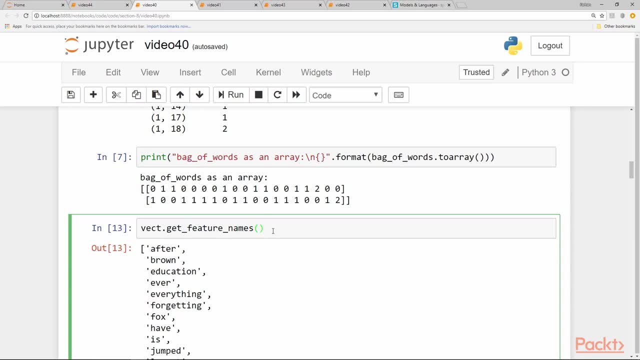 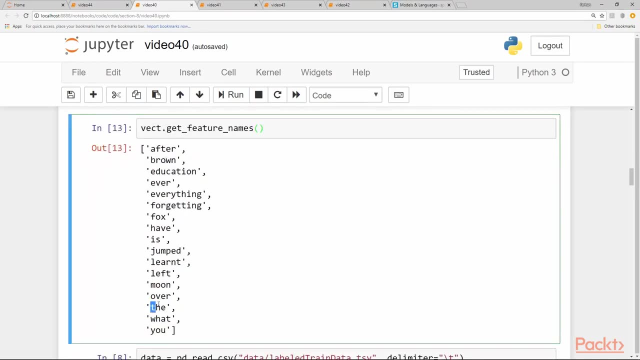 by get feature names function, which is available in our vocabulary too, in the vectorizer. So here we get a list of all the features, all the unique words, at the proper indexes. So the occurs at the 16th index of this list. Let's apply this bag of. 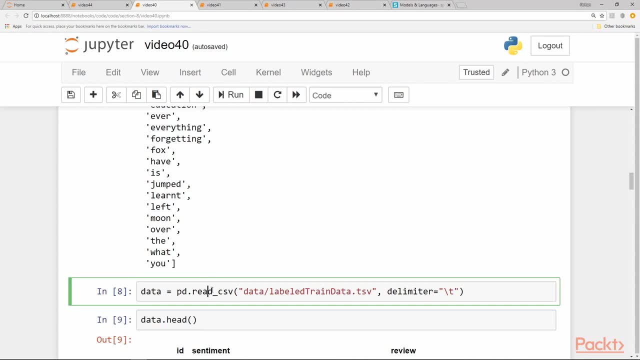 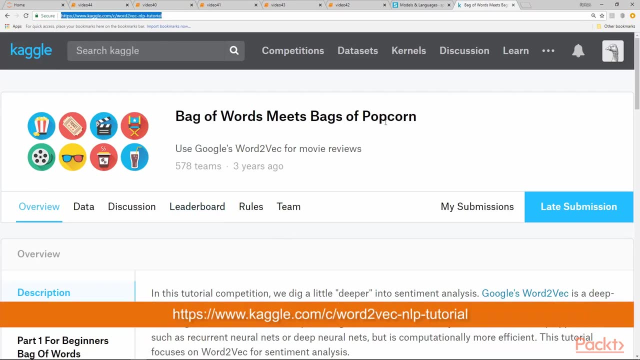 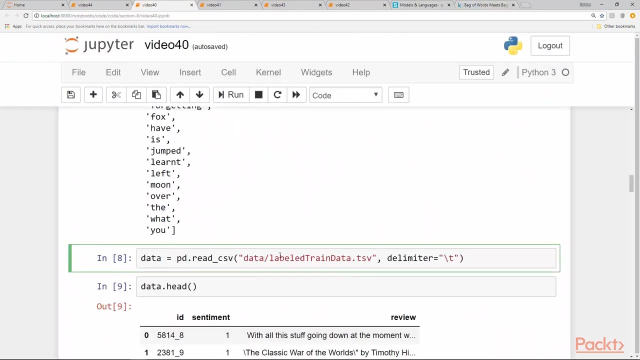 words model to our IMDB movie dataset. So the IMDB movie dataset is available on this URL. bag of words meets bag of popcorn And you can download the dataset from this link. I already downloaded the labeled train data dot TSV, So this is the tab separated values. 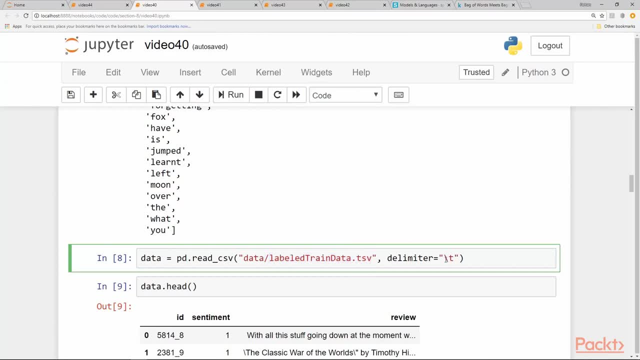 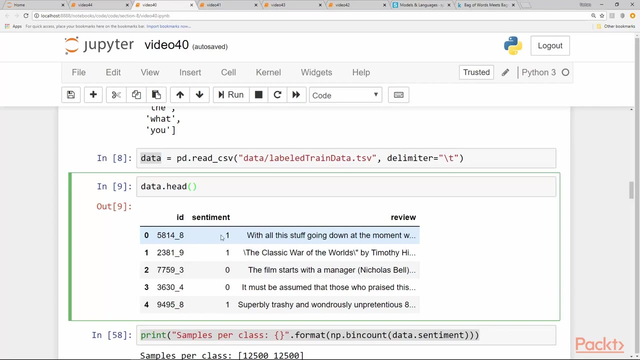 TSV stands for. So that's why we use the delimiter as backslash T instead of comma, which is the default delimiter for read CSV, And we get a data frame back. So let's look at the data frame. So it has an ID, which is the ID of the movie that we're talking about And the 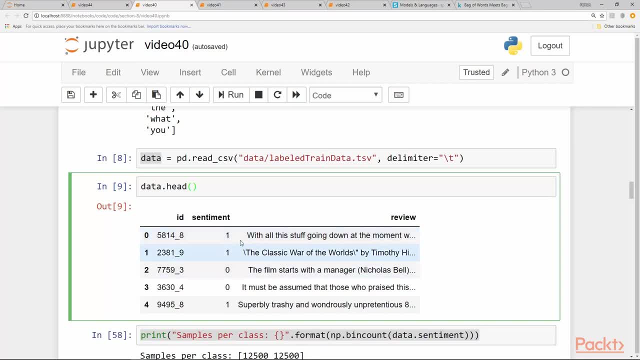 sentiment is either a one or zero. One means positive sentiment, So the text is giving up a positive sentiment. So the text is giving up a positive sentiment, So the text is giving a positive review to this movie. And zero means that the text is giving a negative view overall. 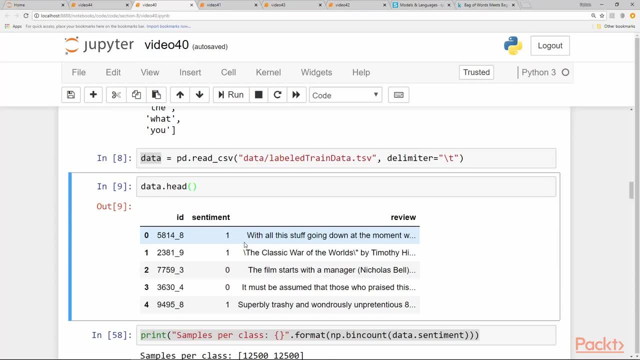 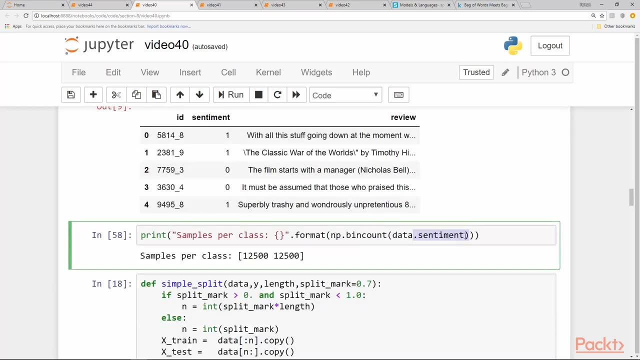 Now, these labels are based on the rating given by the user, So any rating of higher than five stars has been given a one sentiment and and five or lower has been given a zero sentiment. If we count the sentiment columns values, we have exactly 12,500 positive reviews and 12,500. 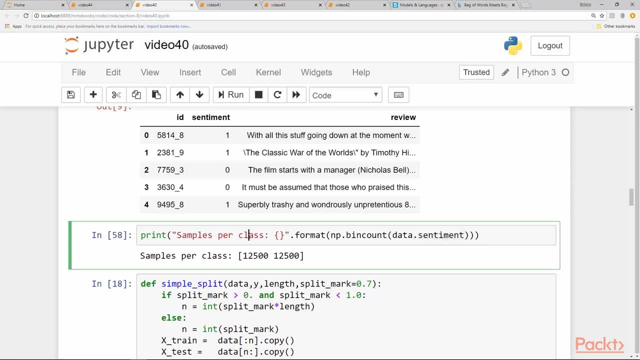 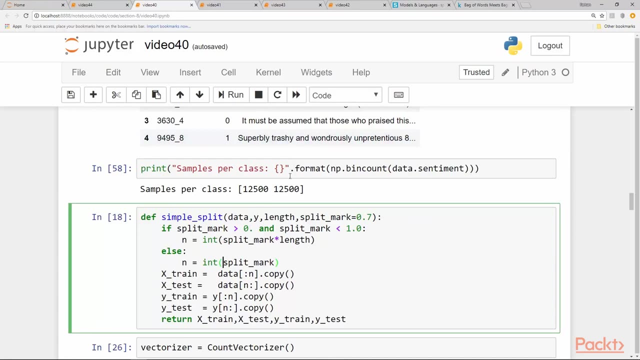 negative reviews. So each class is evenly balanced. So, first of all, it's a classification problem And we are given a sentiment as a label and it's a binary classification problem. Instead of using our normal train test split just for the practice, just let's write a simple split function. 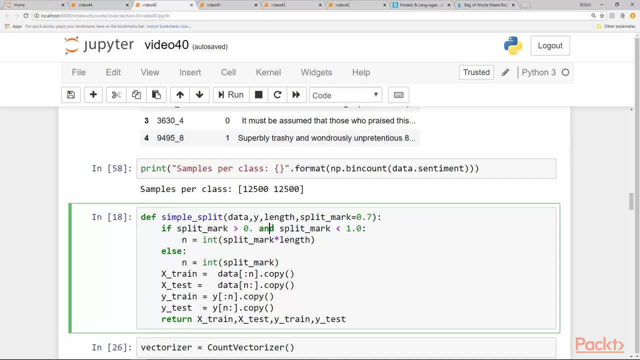 which just divides the data set into default 70-30 split. We have a split mark here, And if split mark is greater than 10, we have a split mark here, And if split mark is greater than 10,, we have a split mark here. 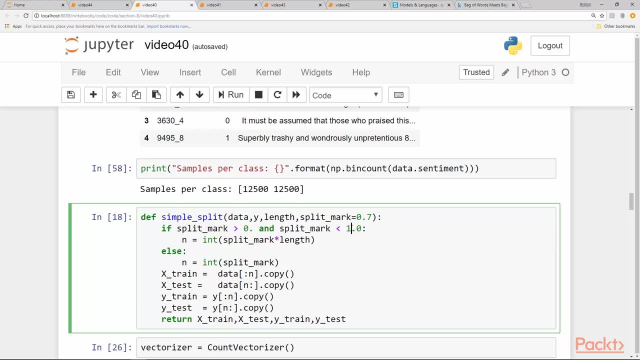 And if split mark is less than zero and split mark is less than one. so we pass a fraction, which then we take it as a percentage, or basically we multiply it by the length of our data set. Otherwise we just convert it into an integer and we split our data from zero to n. 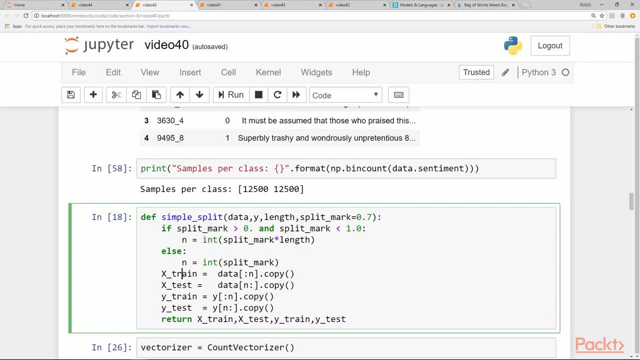 which is calculated here and we return a copy of it as a strain. Now, x test is from n to n, the y train is again from zero to n and y test. We return all this for splits of for x and y. 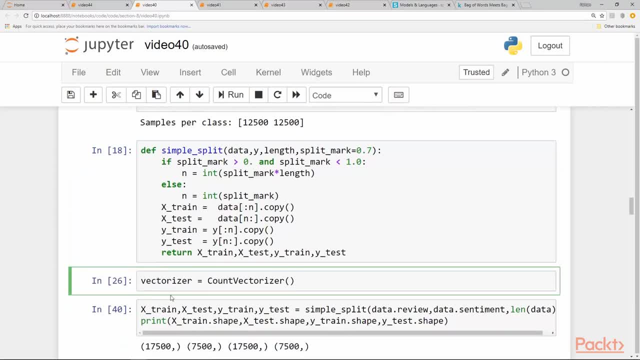 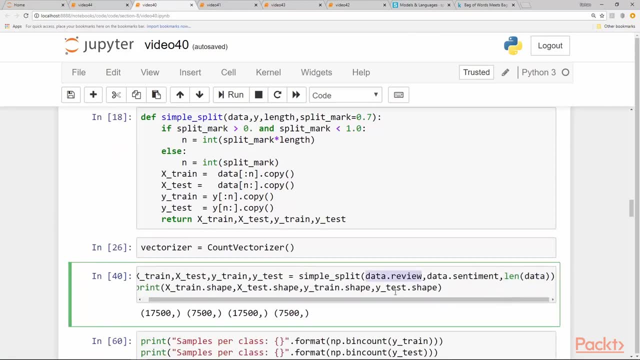 So we initialize a count factorizer as before. we split using simple split. we pass the length and the rest of default values. So we past data dot review column, which is the actual data we want to analyze, And we pass sentiment as our y value. we get this split. 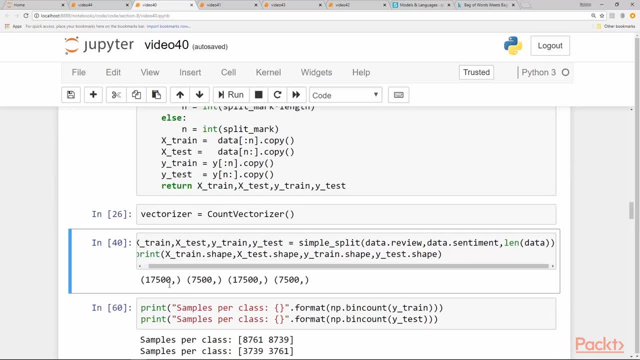 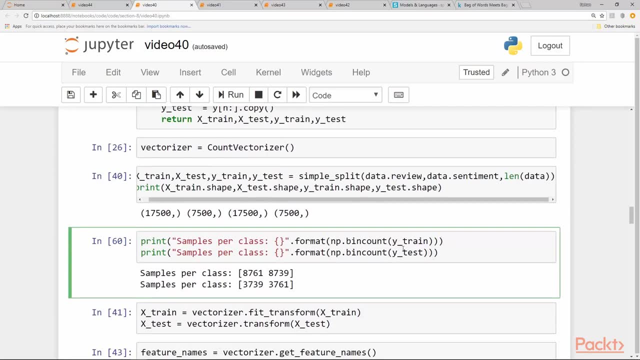 17,500 and 7,500, so we have 25,000 movie reviews and in our splits we have wire train wire test. we have these are the positive and negative classes, which are pretty much balanced state, so we don't really have to worry about it. and the next thing is we fit and transform at the same time our 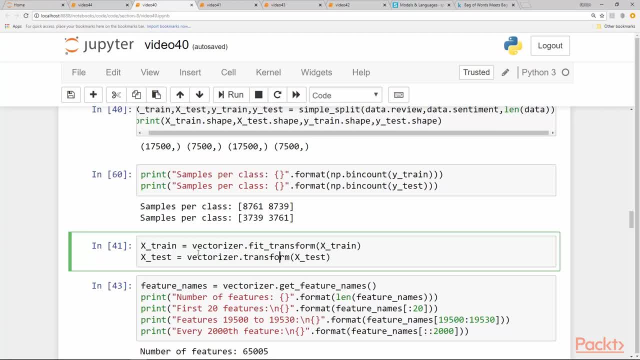 training set and we only transform after the fit has been done to our test set. so basically we have built a vocabulary from the training. the idea is to actually learn all the vocabulary words from the training set and then apply the transformation to build the bag of words on the test set as well. 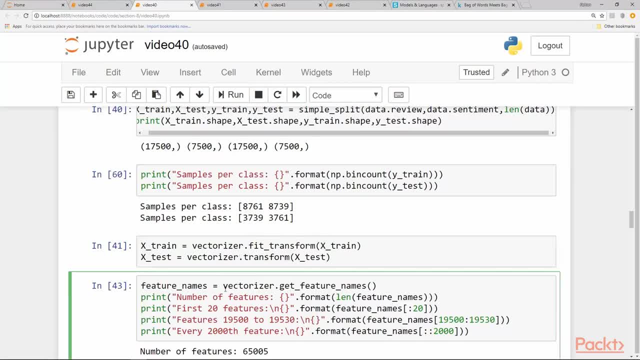 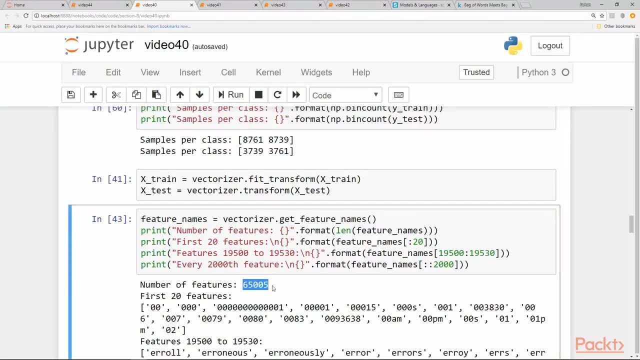 as transforming the training set, of course, and we print the feature names. so we have number of features: 65 0, 0, 5. these are the unique words that we have and the first 20 features we print out. then we randomly print out from nineteen thousand. 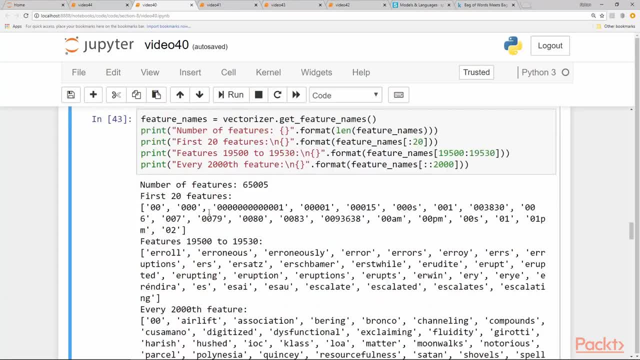 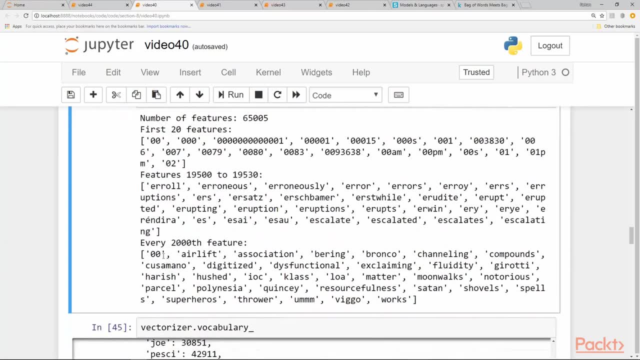 five hundred to nineteen thousand five hundred thirty. initially these are only numbers and or like these: 0, 0, pm and so on, and then every two thousand feature. if you print them out we get these different type of words. so we can see we have successfully built the vocabulary and you can. 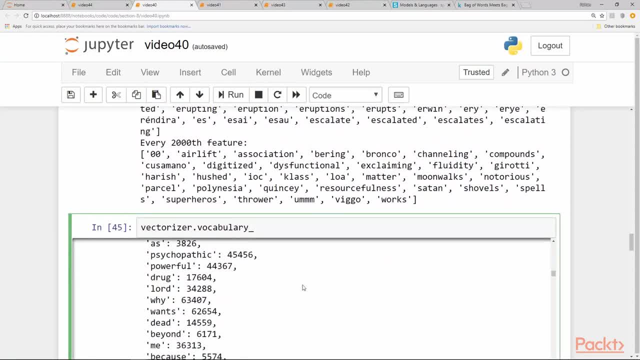 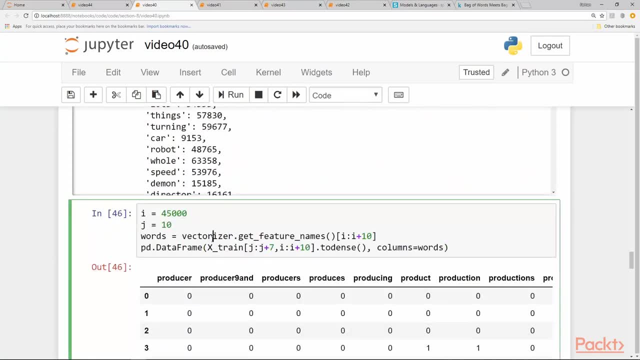 just even print the vocabulary to just see the counts of in our dictionary of each word, if you want to see if if a particular set of words is printed, then you can just print the vocabulary of words occur in our data anywhere. we can just pick randomly some number, some index and we 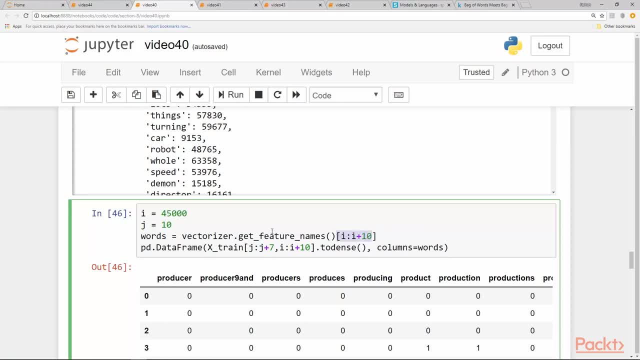 extract the features, like, for example, ten features from this index, for example, like forty five thousand, as we have sixty five thousand features and we take the ten rows of the data from X, train, J to J or other seven rows from the data, starting from the tenth row and the 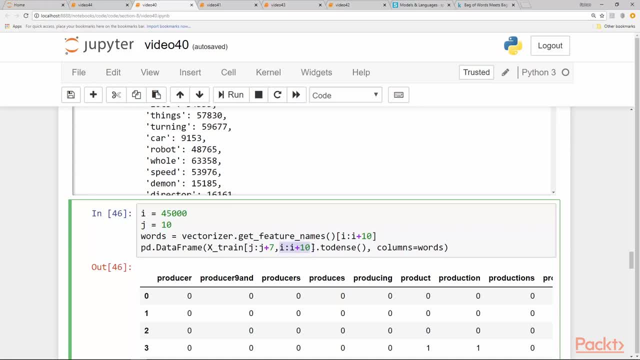 columns which are representing features, or sixty five thousand features. we pick the only the ten columns starting from forty five thousand to forty five thousand ten and we convert that slice into dense a and we create a data frame using the words we extracted from the feature names. this is: 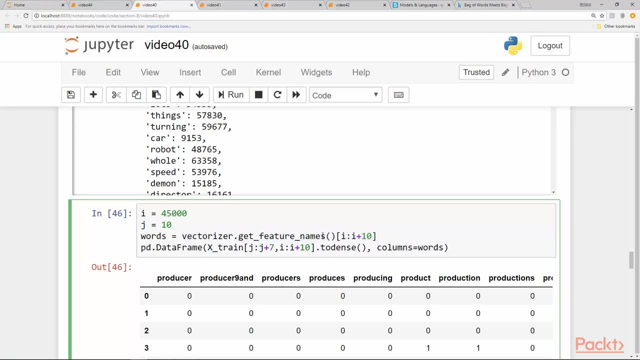 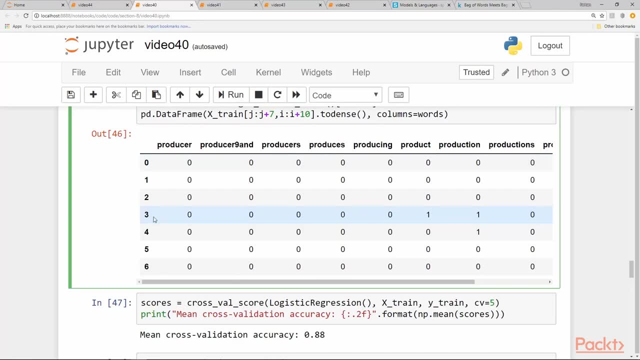 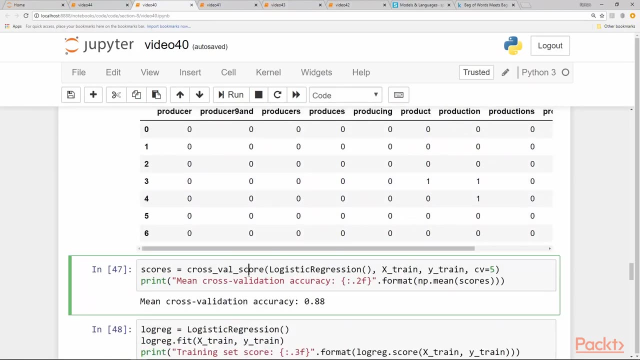 a particular set of words. we are interested in whether this it occurs in this slice or not, and we can see that production of occurs in this slice as this index and also in the index 4, and the rest are pretty much 0.. The next thing we are going to do is we're going to use, since it's a binary classification problem, 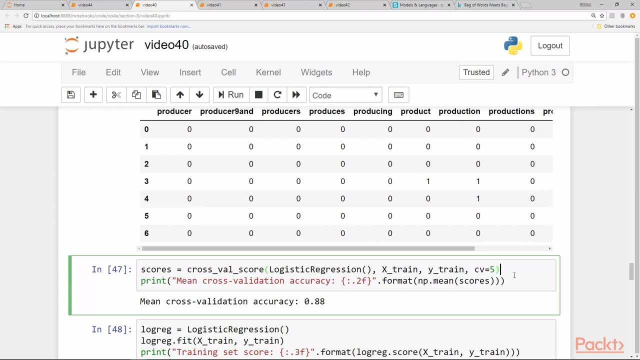 so it's natural to use logistic regression first for it. and using logistic regression we do a cross validation score with cv equal to 5 and our mean cross validation score, which we pre-calculate from the mean of scores, we get a 0.88.. So it will take a little bit of time, like. 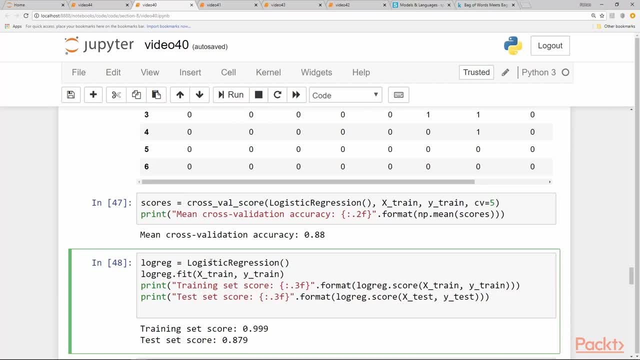 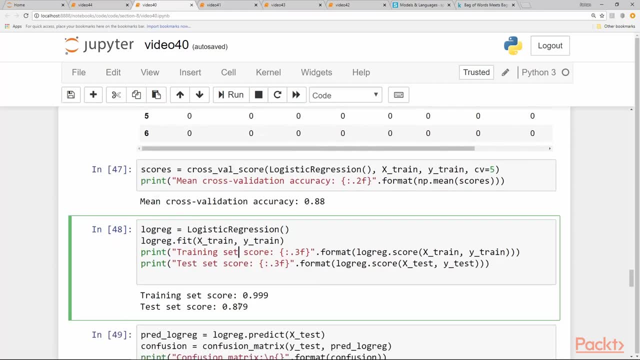 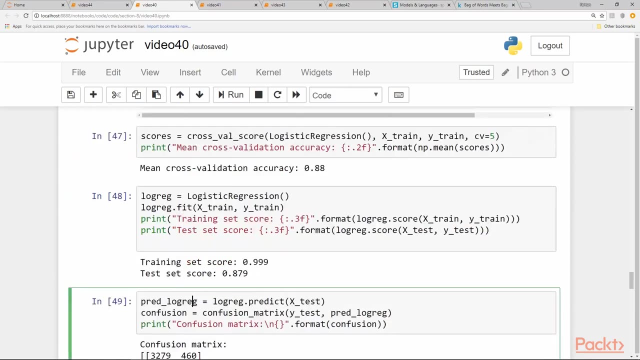 a few minutes Now. let's create a logistic regression model with default values and see if it is consistent with our cross validation score, and so on the test set, we can see that we have a 0.87, which is consistent with the cross validation score 0.879.. We can print the confusion. 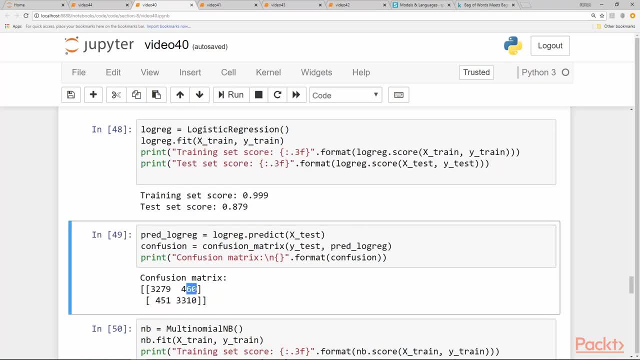 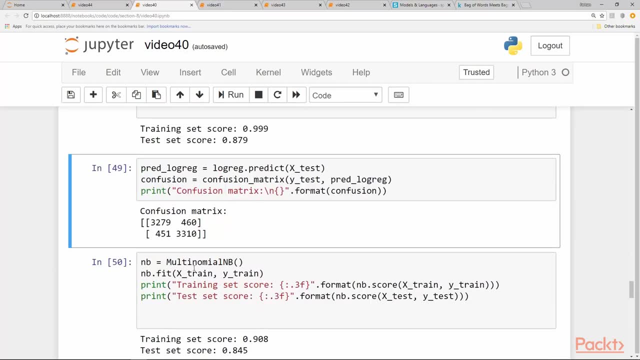 matrix. So we can see there are four: 460 false positives and 451 false negatives, So we have mid 400s incorrect in both cases. We can also try a multinomial naive Bayes, which is another variant of naive Bayes model that we have used before. we before used the Gaussian naive Bayes We have briefly discussed. 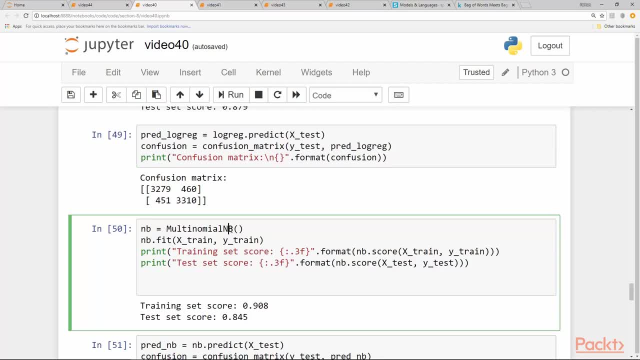 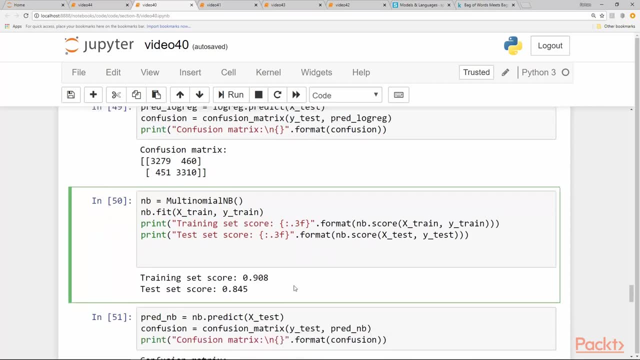 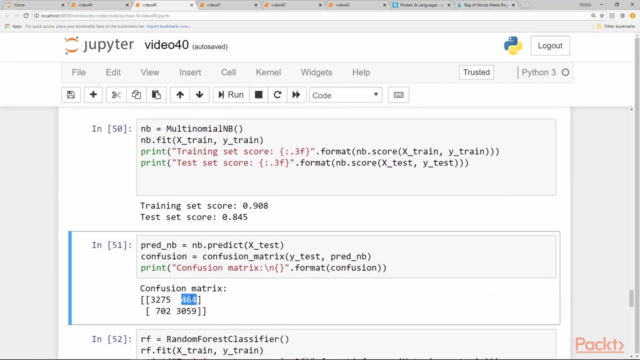 what naive Bayes is and makes a naive assumption about independence of the features and it's based on the Bayes theorem And all we get a 0.845 test score which is lower than logistic regression and our confusion matrix kind of matches the false positives, but on the false negative side it is is much worse. 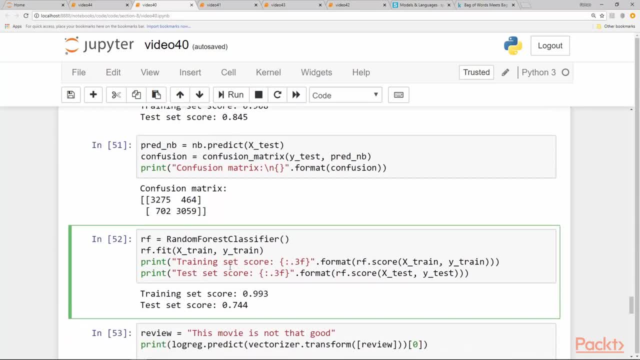 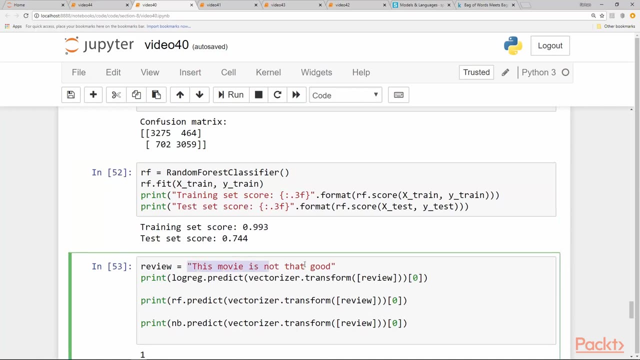 And similarly for the random forest classifier with default number of trees, we only get 0.744, which is significantly lower than logistic regression and naive Bayes both. And now let's do some predictions. We just create a review, just a simple movie review, and we say this movie is not. 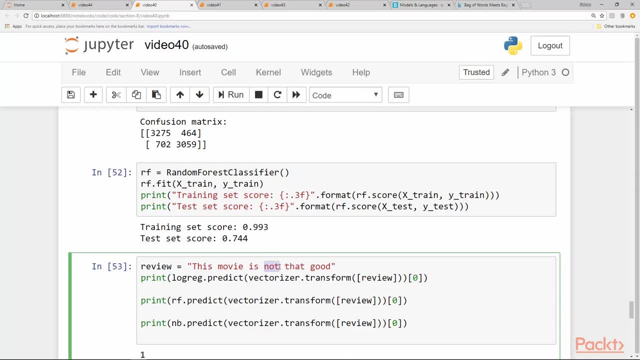 that good. Just notice that we have two words here: not and good, and separated by that. So this more review is obviously bad. It's a negative review. The sentiment is negative And if we just convert it using our vectorizer and we use it to predict our sentiment using the trained model of a logistic 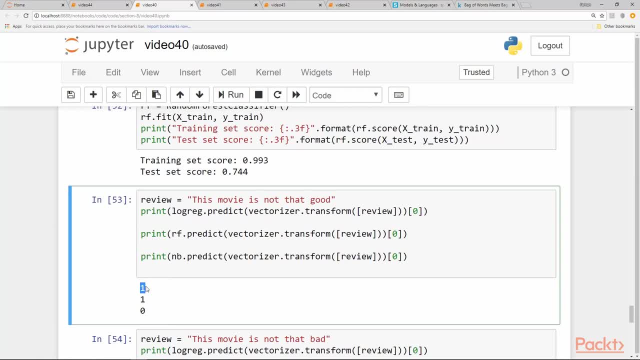 regression model says that it's a positive review, which is wrong. Our random forest model says also it's a positive review, whereas naive Bayes says it's a negative review. So the naive Bayes was able to pick it correctly this time. for our synthetic sentence, Let's try another one. This movie is not. 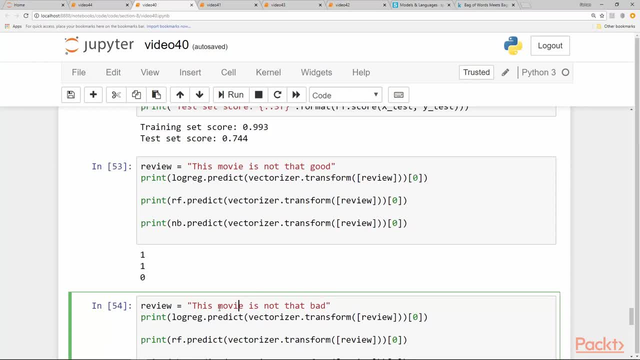 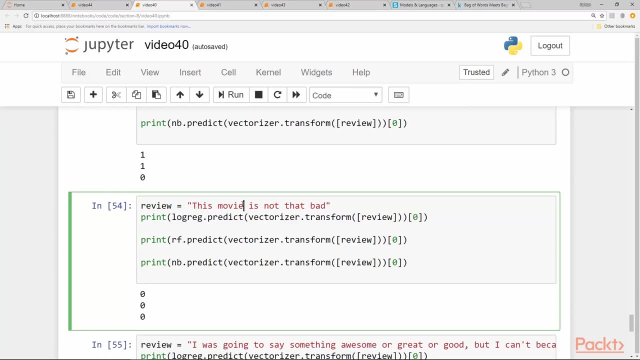 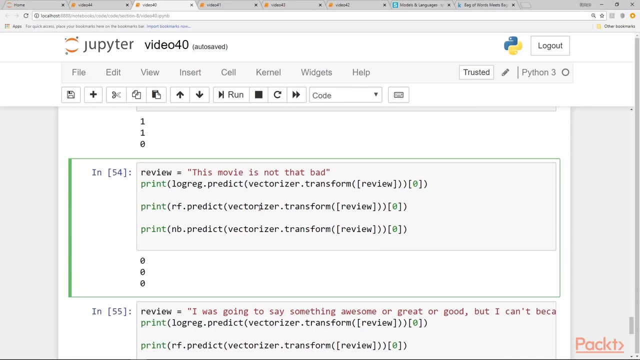 that bad. In this case it's a positive review. at the end of the day, All of our models say that it is a negative review, So they were fooled by the words again. So you have to get this insight into overall how these models actually are predicting and by just doing these simple thought, experiments and experimentation. 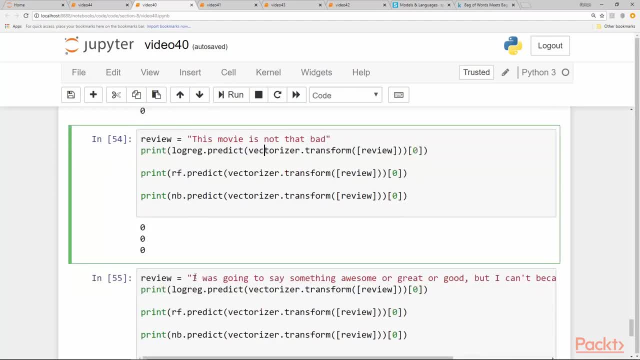 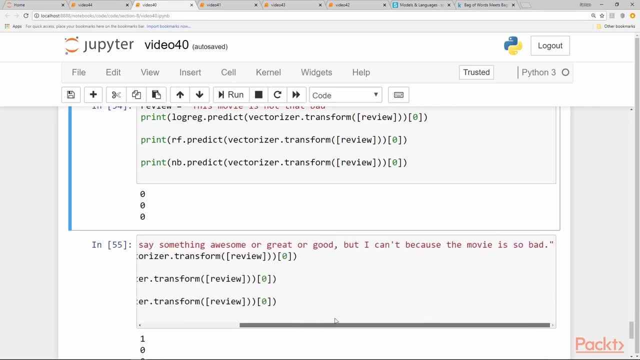 with test or dummy reviews. And lastly, look at this sentence. I was going to say something awesome or good or great or good, but I can't because the movie is so bad, So obviously it's a bad review, So the answer should be zero. 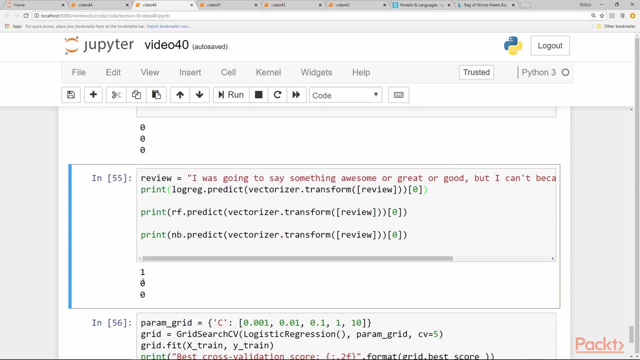 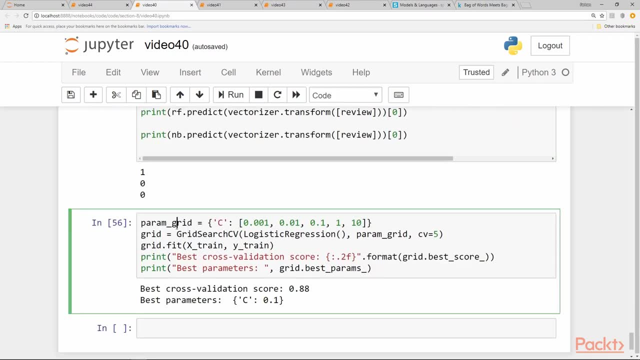 Again, our logistic regression model was fooled by this, but our random forest and naive Bayes were able to correctly identify it. The last thing we can do before we end this video is to have a grid search using logistic regression, with the C parameter for starting from 0.001 to 10, varying it like in about. 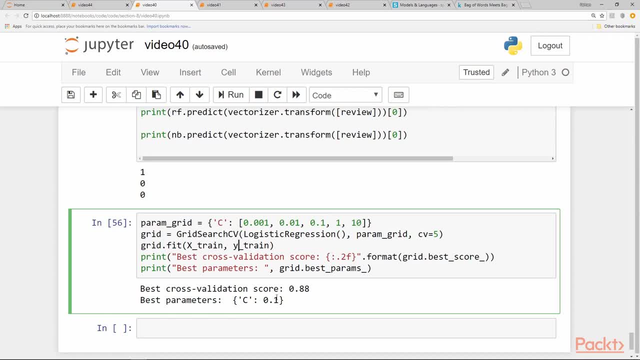 five values. If we do this, it will take a while, but we get a cross validation score from grid search, CVS: 0.88, and the C value most appropriate C value which gives us the highest score, is 0.1.. So we have trained a logistic regression model. We have done some experimentation. We see that even if our 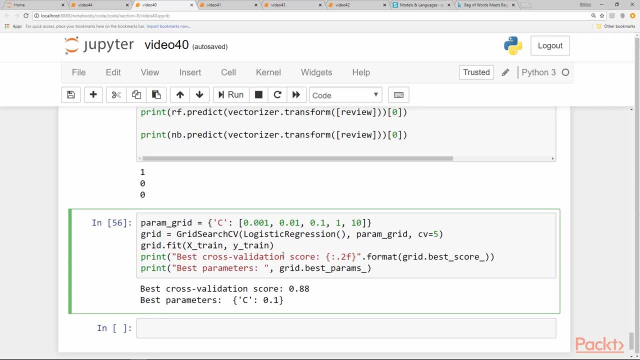 model is as high as 0.88, it doesn't mean that it's really going to predict everything correctly. Just by creating some synthetic sentences, we can see that our best model also fails in many cases. Thank you for watching.